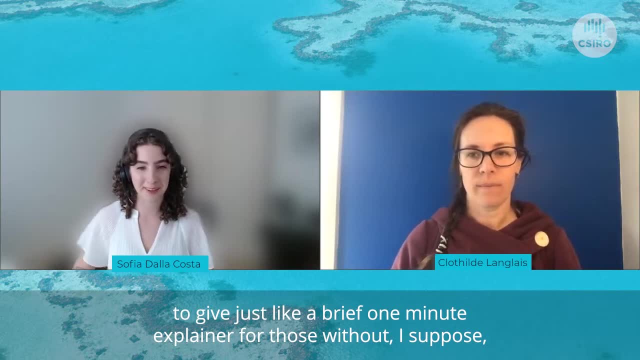 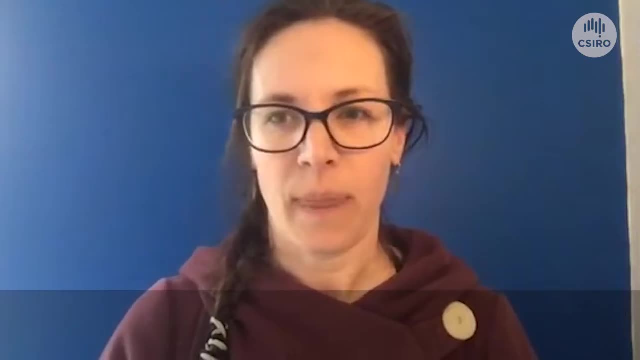 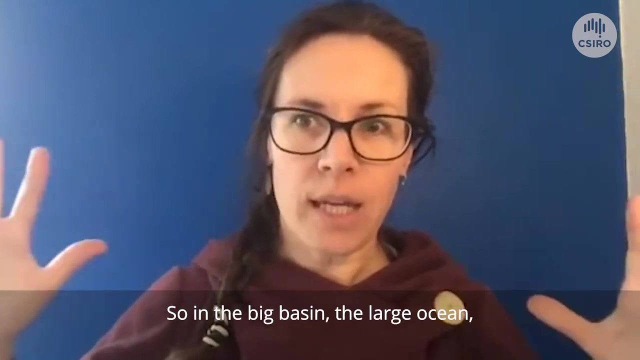 is it possible for you to give just like a brief one minute explainer for those without, I suppose, a science background and who don't know much about how oceans work? Yes, so the easiest way to explain ocean current it's more at very large scale, So in the big 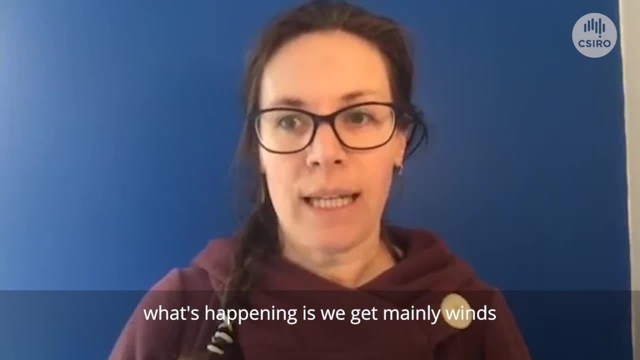 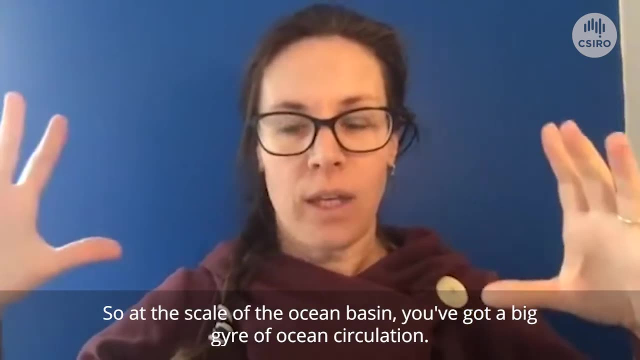 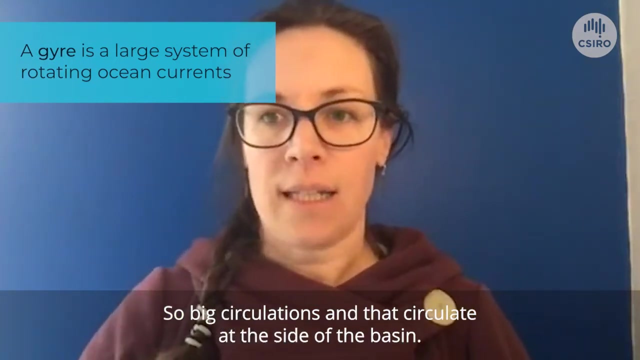 basin, the large ocean. what's happening is we have many winds that are driving the ocean circulation. So at the scale of the ocean basin you've got big gyre of ocean circulation, so big circulation in that circulate at the side of the basin and that's really due to the wind. 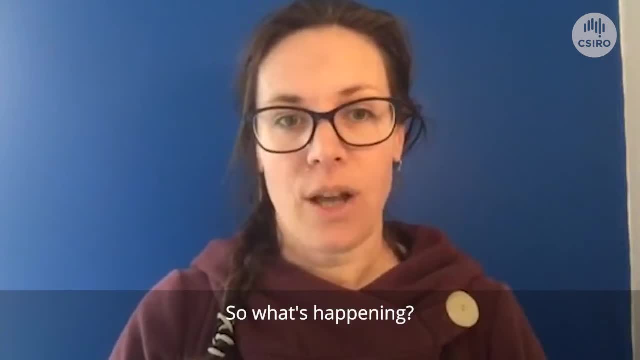 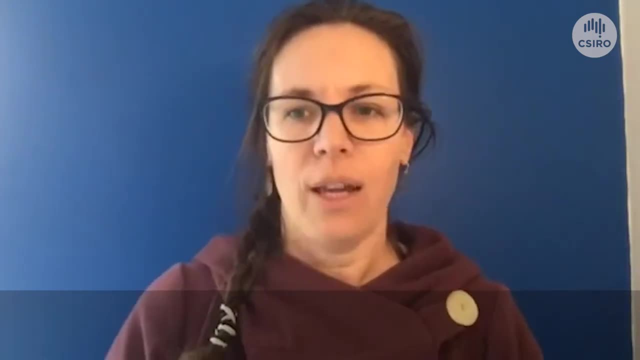 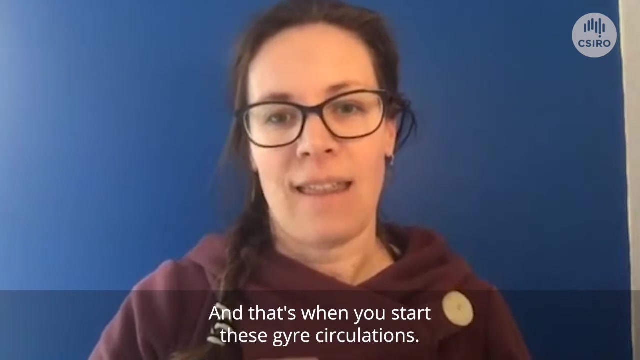 forcing In part. so what's happening? you've got those big westerlies around the 40 degree north or 40 degrees south and they're going to try to push the water in one way or in another, and that's when you start this gyre circulation. So in the northern hemisphere it's going to be in a 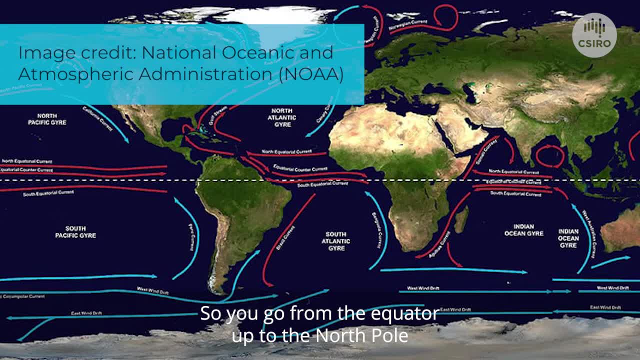 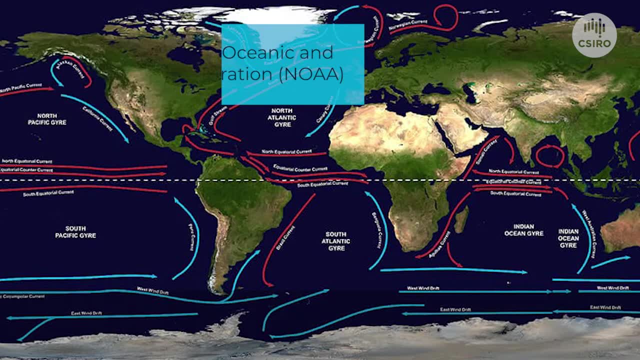 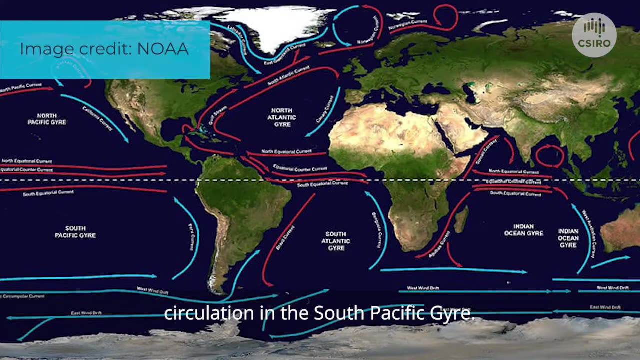 clockwise circulation. So you go from the equator up to the north pole and then you go in a clockwise circulation all around Closer to Australia. so in the south Pacific what's happening is you've got an anti-clockwise circulation in the south Pacific gyre, So you've got warm water coming. 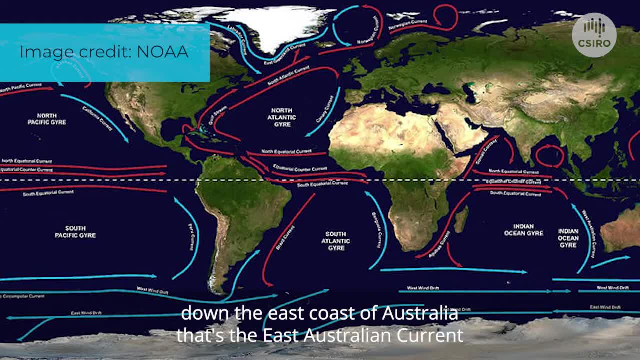 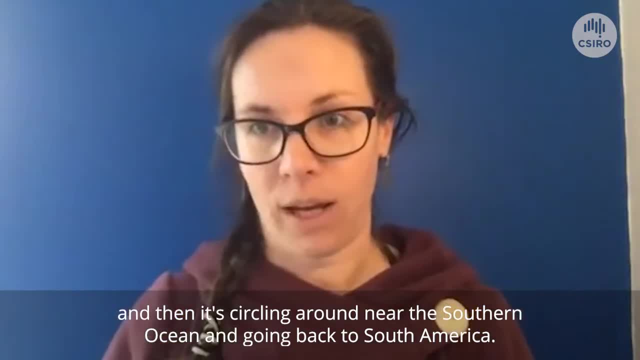 along the equator and then going all the way down the east coast of Australia- that the east Australian current- and then it's circling around near the southern ocean and going back to South America. So that's a large scale gyre circulation. 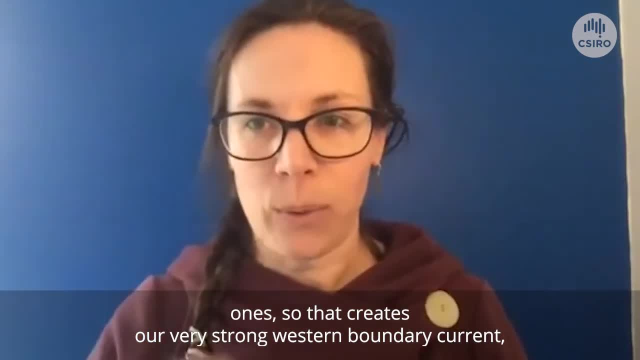 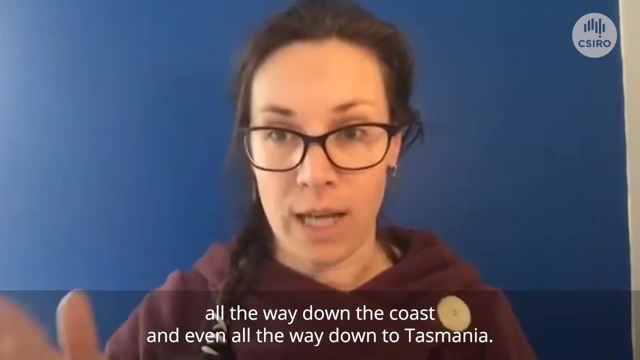 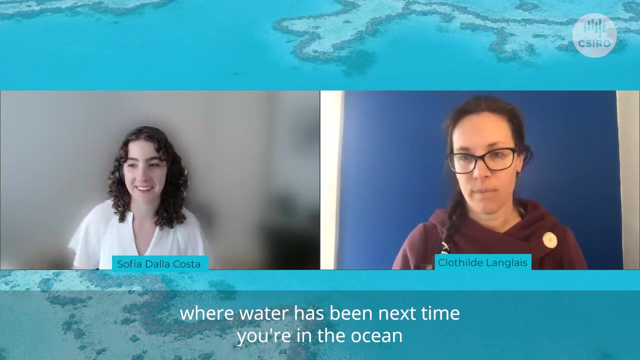 And those ones so that create our very strong western boundary current, which for us is the east Australian current, and bring warm water all the way down the coast and even all the way down to Tasmania. Wow, I think that's really interesting to think about Where water has been like. next, 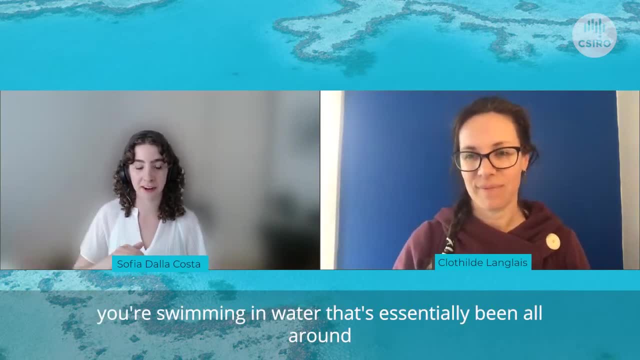 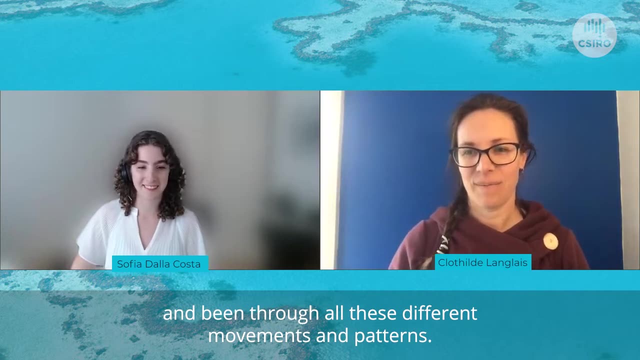 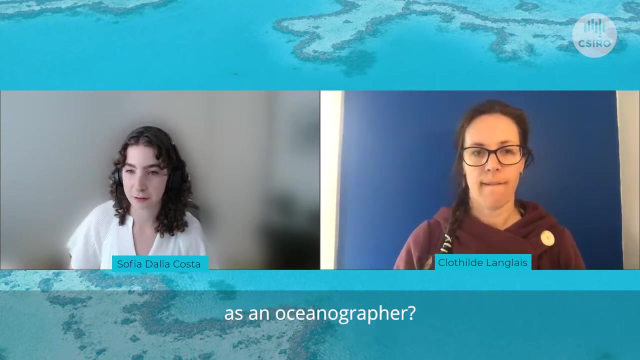 time you're in the ocean, you're swimming in water. that's essentially been all around Australia and it's come from all these different and been through all these different, I suppose, movements and patterns. It's really interesting. Yeah, So can you take us through, I suppose, a day in a life as an oceanographer? 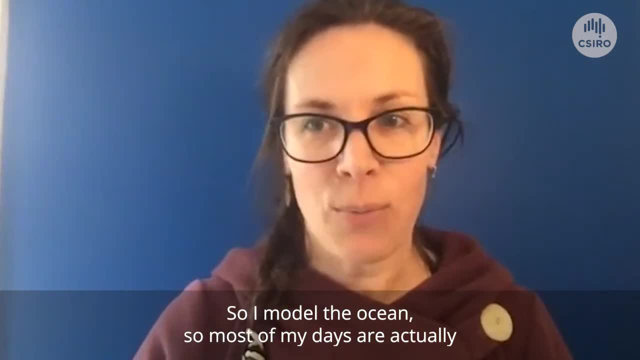 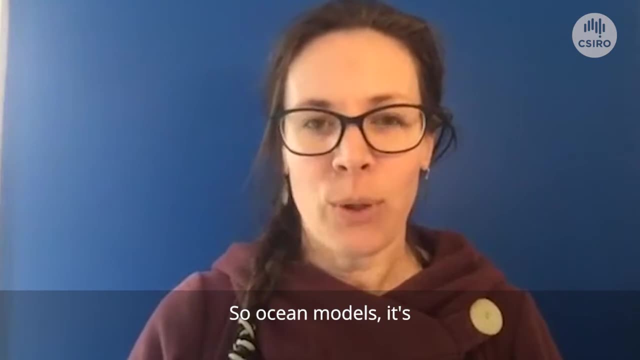 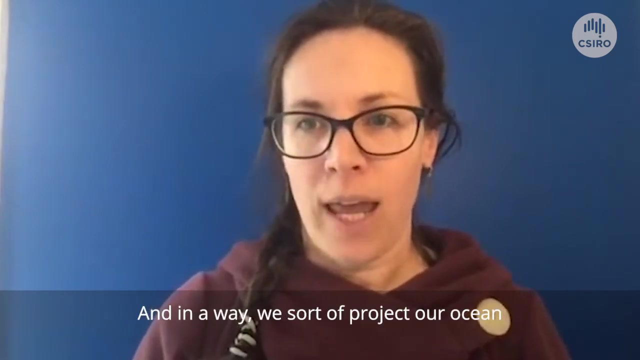 So I model the ocean. So most of my days are actually in front of my computer looking at ocean models. So ocean models: it's a tool we use to mimic the ocean circulation And in a way we sort of project our ocean onto a grid And on this gridded ocean. you look at the evolution of current and temperature and salinity. So if you're interested in the global ocean, often our grid is the size of 10 of kilometers or so, because we can't go higher resolution, We don't have computers that are performant enough. 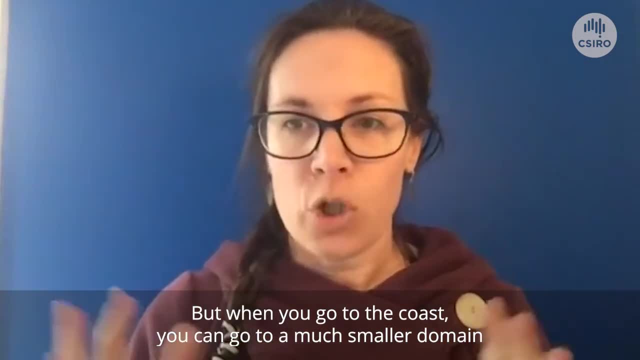 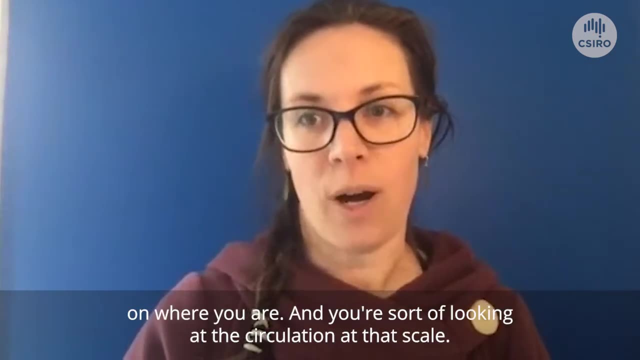 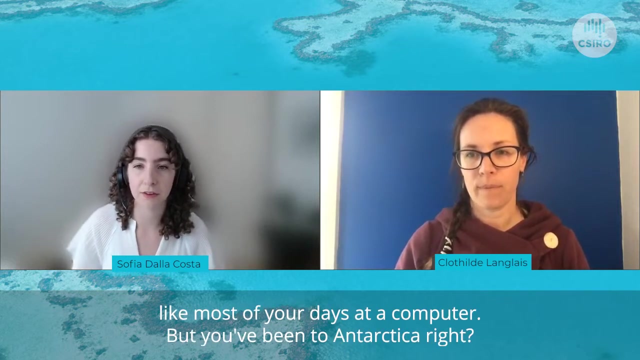 But when you go to the coast, you can go to a much smaller domain and then you can start to go to 10 or 100 meters resolution, depending on where you are. So you're looking at the circulation at that scale. So you've spent, as you say, like most of your days at a computer, But you've been to Antarctica. 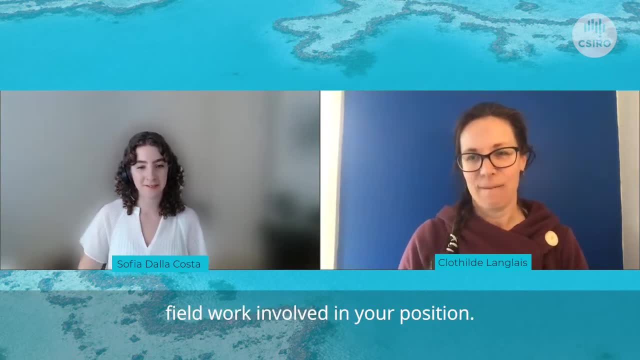 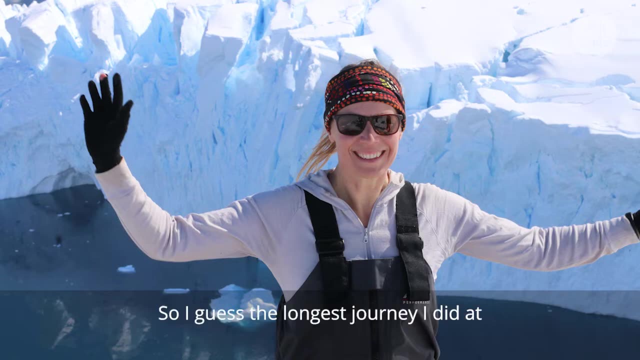 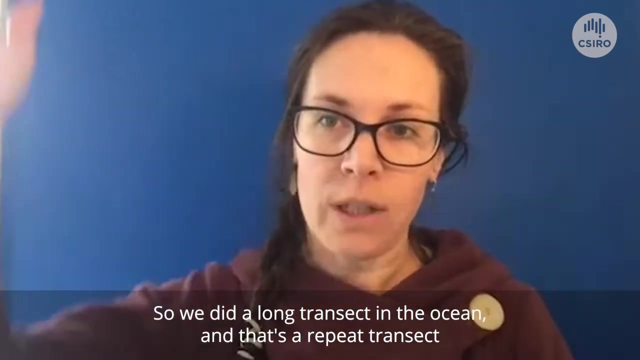 right, There's still some real work involved in your position. Yeah, So I've been helping all the observationalist colleagues as well, So I guess the longest journey I did at sea was during a campaign. we need to go to the equator, So we did a long. 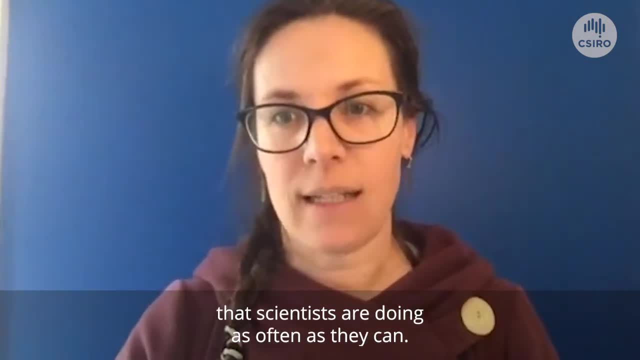 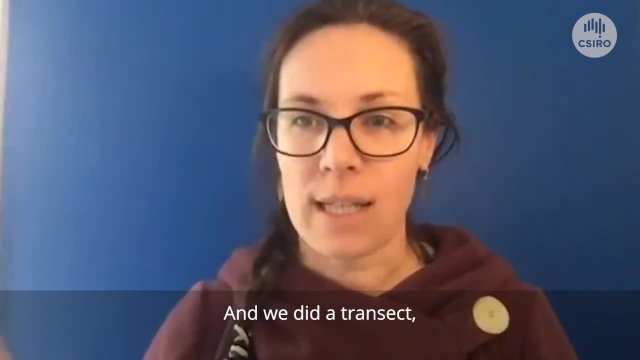 transect in the ocean And that's a repeat transect that scientists are doing as often as they can, And then they share the information across the international community And we did it transect And during that time, usually working shift, shift work. 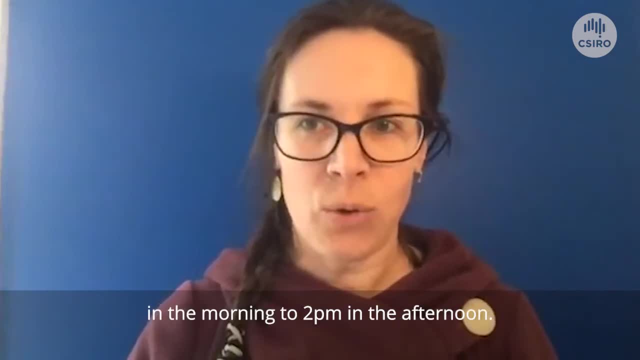 So I was from 2 am In the morning to 2 pm In the afternoon, And then there's another team, you know, catching up 2 pm In the afternoon all the way to 2 am. 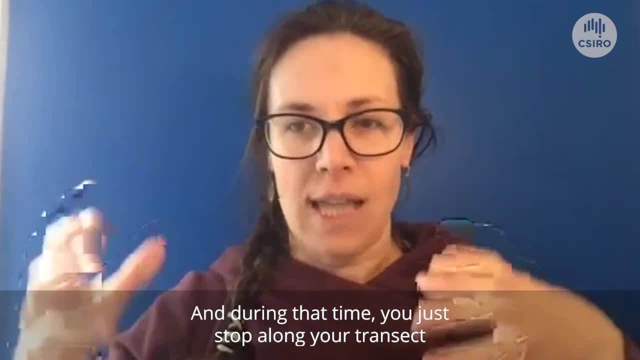 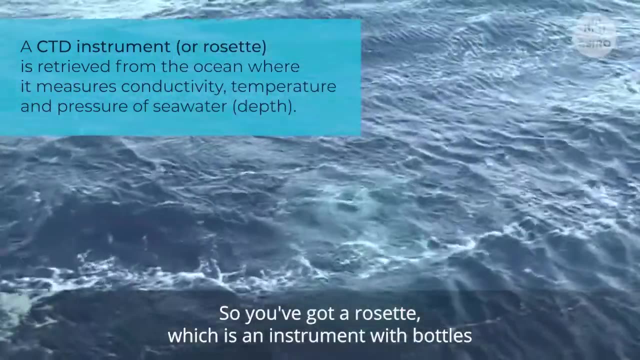 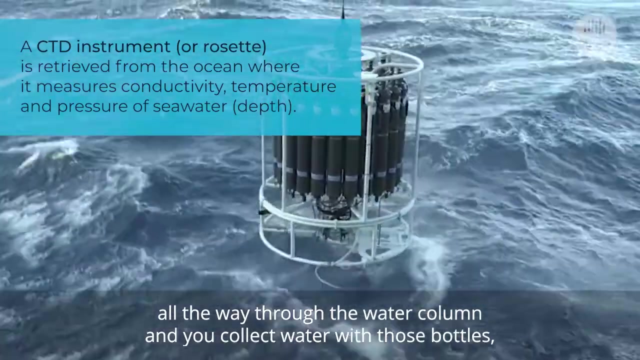 In the morning, And during that time you just stand, you do stop along your transect and you try to sample the ocean all the way down to the bottom. So you've got a rosette, which is a instrument with bottle that you drive all the way through the water column and you collect water with those bottles. 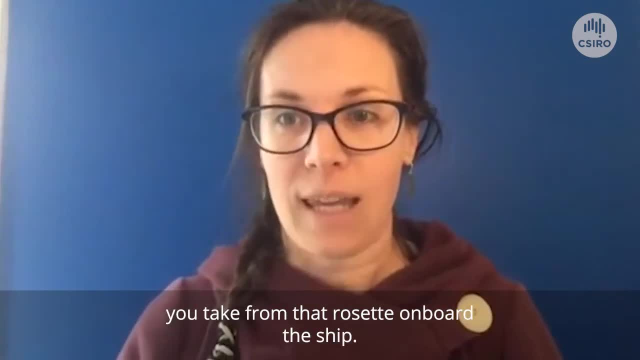 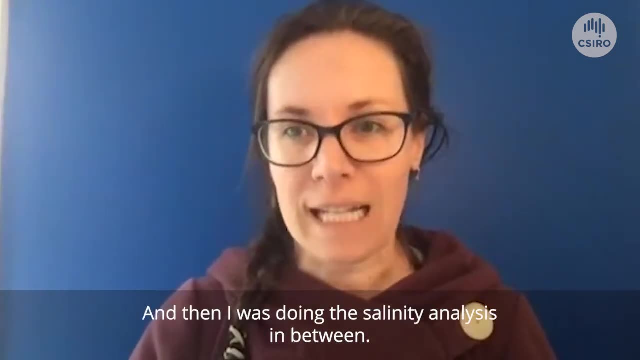 And then you analyze the water sample you take from that rosette on board the ship. So my job was to help with the rosette collecting the water And then I was doing the salinity And then I was doing the salinity analysis in between. 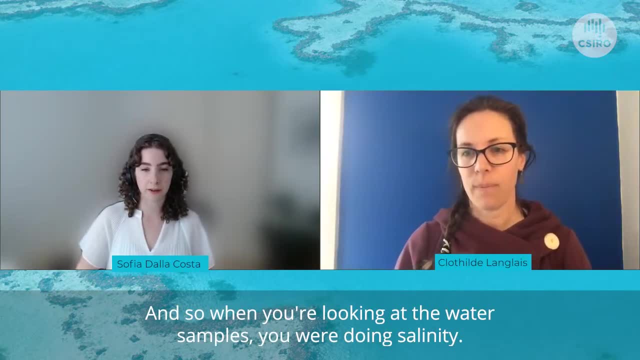 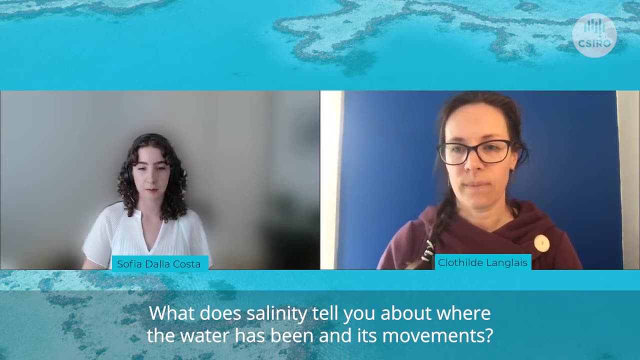 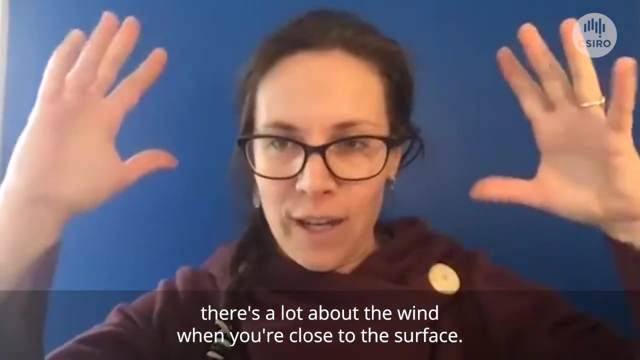 Yeah, okay, And so when you're looking at the water samples, you were doing salinity. What does salinity tell you about where the water has been and its movements? So, to understand the movement of the ocean, there's a lot about the wind when you close to the surface, when, when you start to go in a deep ocean, it's becoming more about the density of the water. 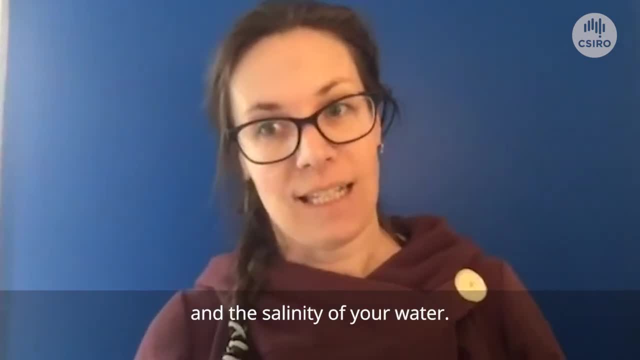 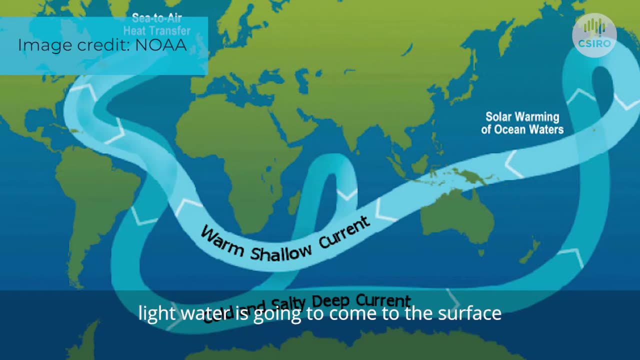 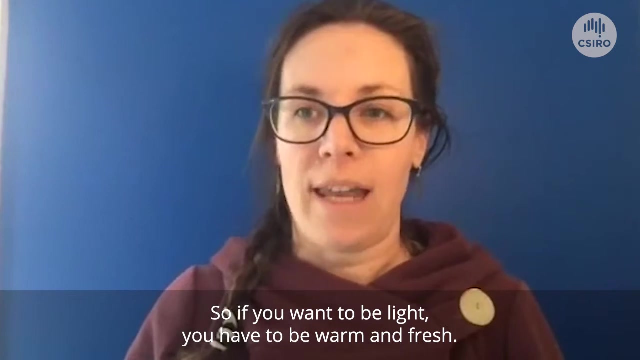 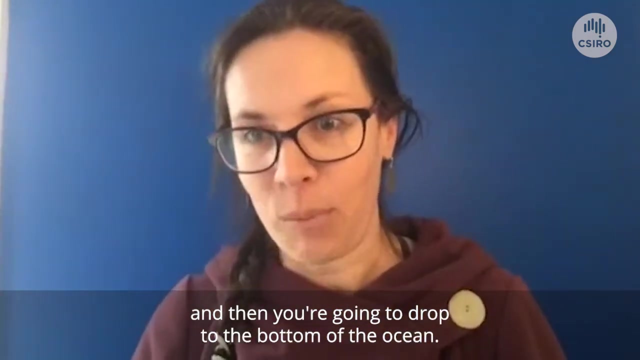 So density is a function of the temperature and the salinity of your water, And so every water is going to go to the bottom of the ocean, where light water going to come to the surface and it's a mix of temperature and salinity. So you need, if you want to be light, you have to be warm and fresh, And if you want to be heavy at the water drop, you want to be cold and salty, and then you're going to drop to the bottom of the ocean. and another thing you trace when you look at those water, sometimes oxygen. 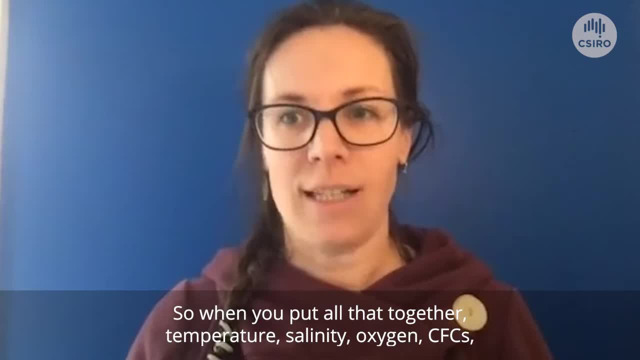 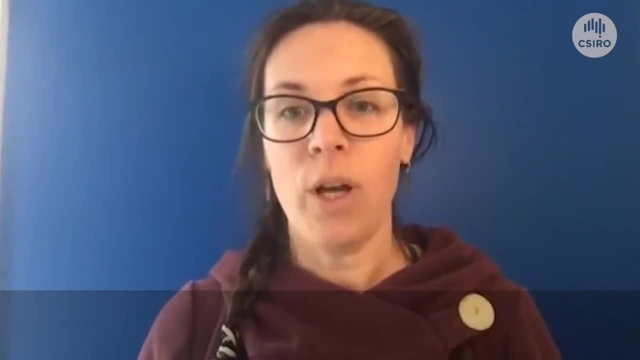 So when you put all that together- temperature, salinity, oxygen- Okay, CFC, you've got that and other information that you can get out of the water sample- You actually can um use your detective work to trace where it's coming from. 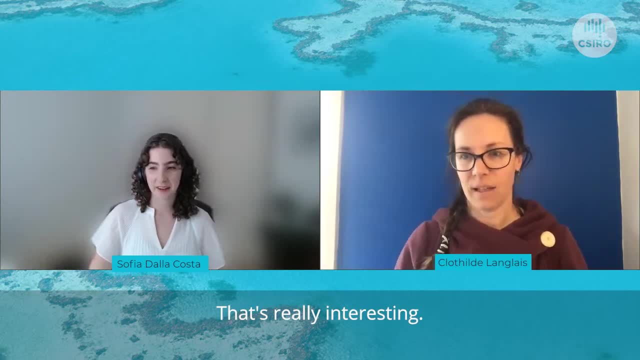 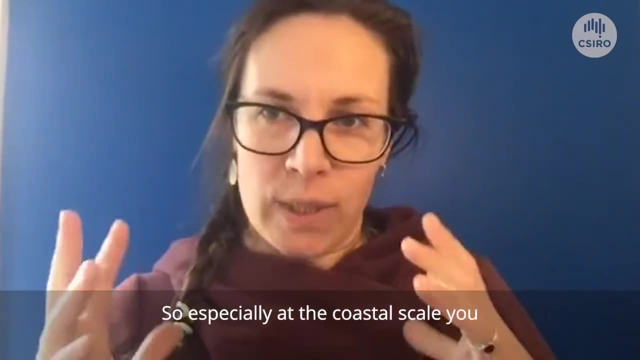 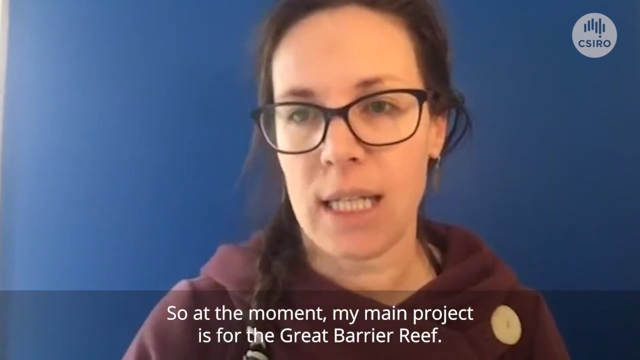 Yeah, that's so cool, That's really interesting. And so what is the link between your research and the broader picture? So, especially at the coastal scale, you always, always and often work in multidisciplinary team. So at the moment, my main project is for the Great Barrier Reef. 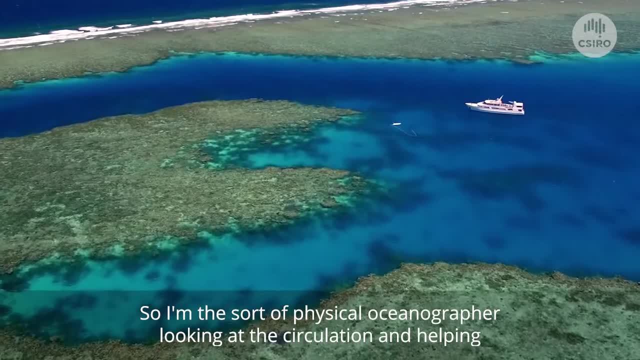 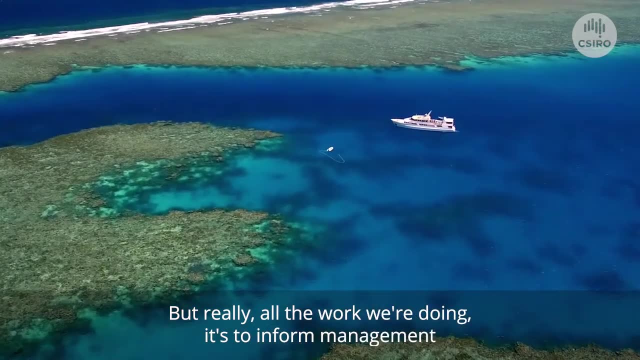 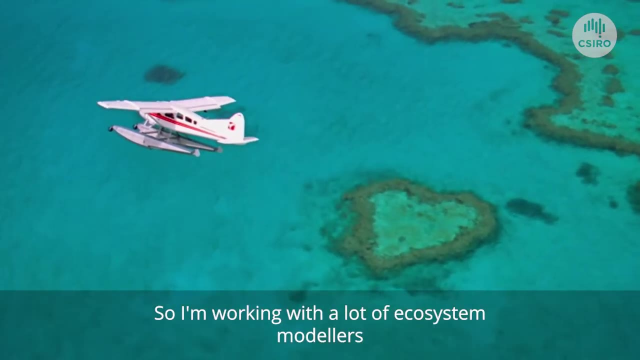 So I'm the sort of physical oceanographer looking at the circulation and helping others understand the connectivity between the different reefs, But really all the work we're doing is to inform management and better management of the reef, um and adaptation. So I'm working with a lot of um, ecosystem modeler and biogeochemist and water quality, people and um. 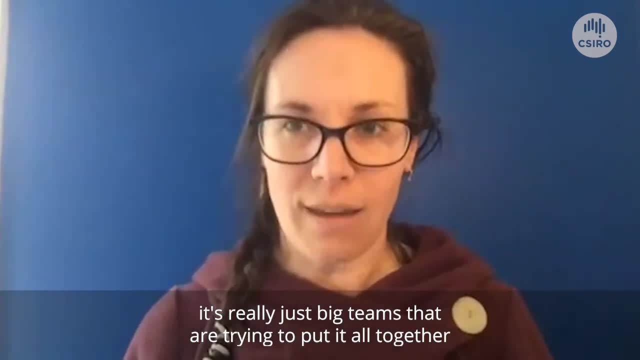 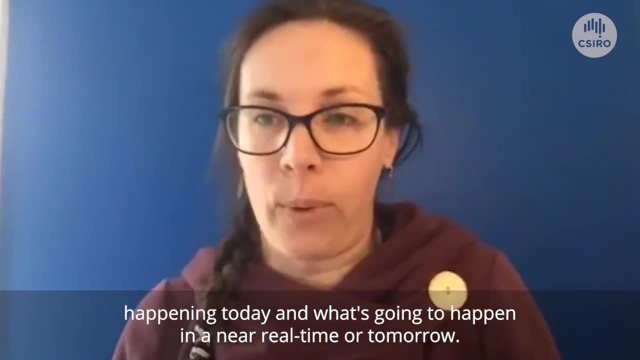 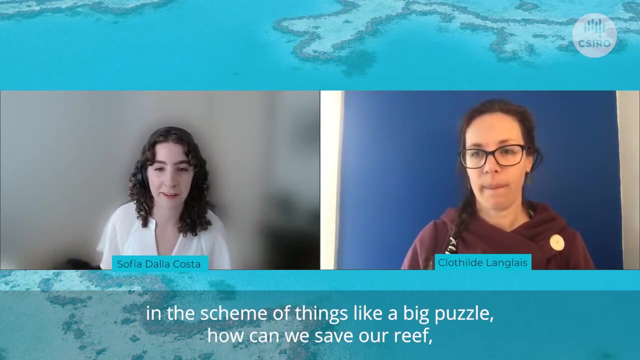 really just big teams are trying to put it all together to improve the health of the reef and try to have a picture of what's happening today and what's going to happen in a near real time or tomorrow. So it seems like, in the scheme of things, like a big puzzle: how can we save our reef? And you're one of those pieces contributing to all the other pieces of research that are going on. 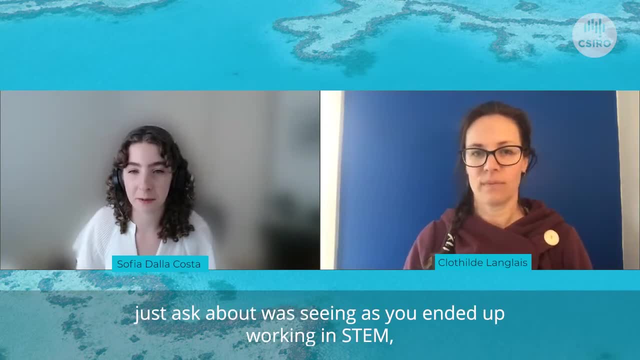 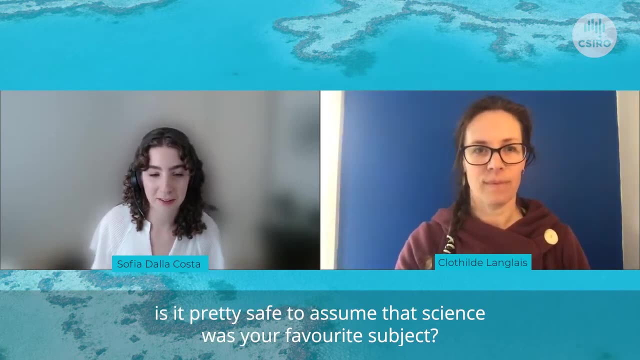 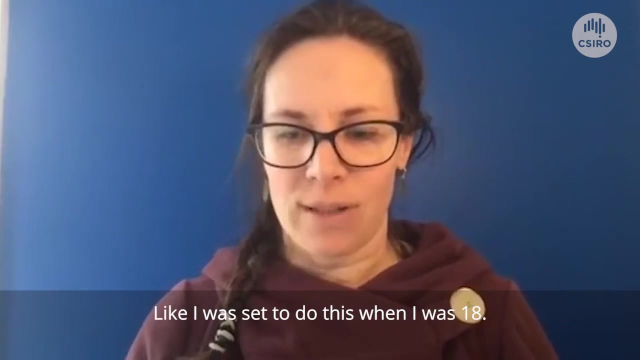 Yes, Great. So the next thing I wanted to just ask about was, seeing as you ended up working in STEM, is it pretty safe to assume that science is your favourite subject? So I sort of knew pretty early that I wanted to become a physical oceanographer, like I was set to do this when I was 18.. so I think it's pretty young to know what you want to do in life. 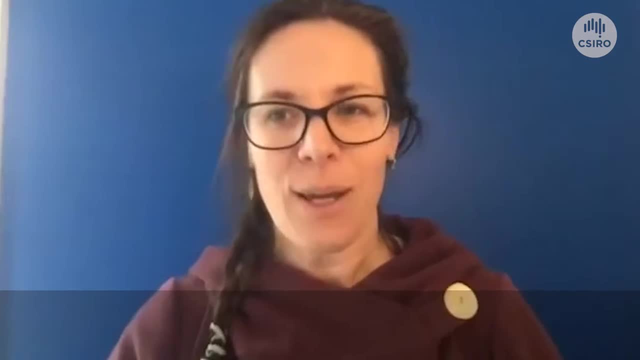 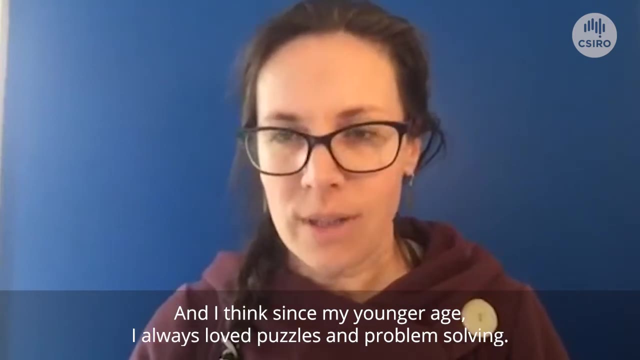 Although I'm pretty sure I didn't know exactly what it entailed completely, but I wanted to become a physical oceanographer And I think since my younger age I always loved puzzles and problem solving, So I guess going more to high school. 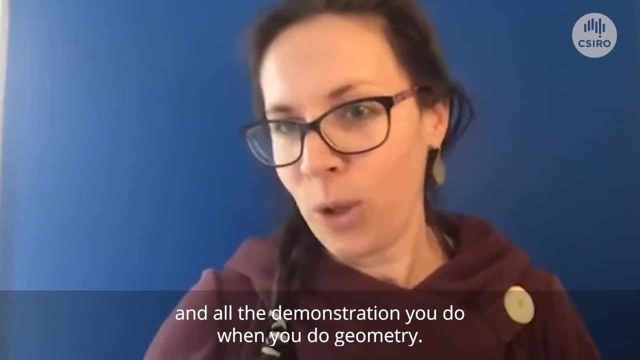 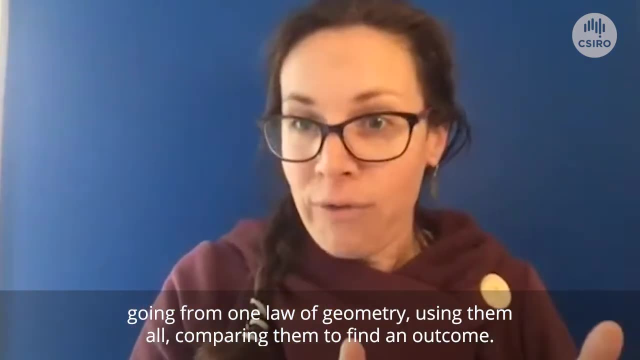 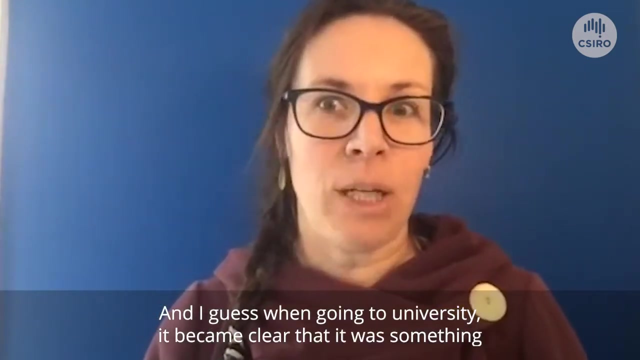 it become German. I love geometry and all the demonstration you do when you do geometry. I love the complexity and the solving of problem, going from one law of geometry, using them all, comparing them to find an outcome, And I guess when going to university it become clear that it was something that you could do with the law of physics. 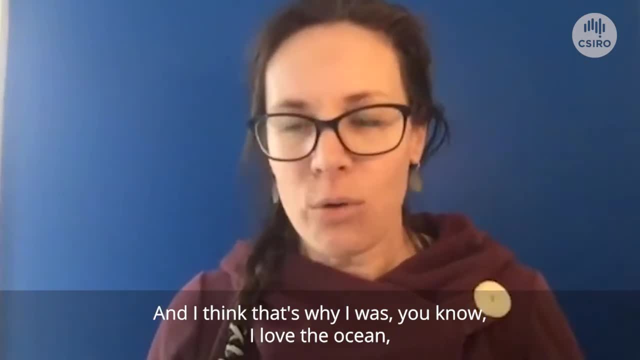 A lot and I think that's why I was passionate. you know, I love the ocean. but a lot of people, when you say, oh, you love the ocean, you're studying animals, Like, oh no, I don't know. 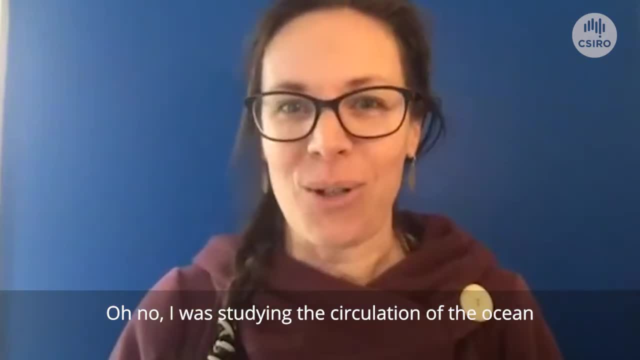 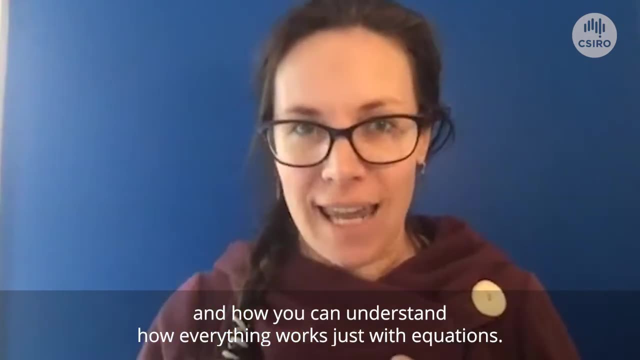 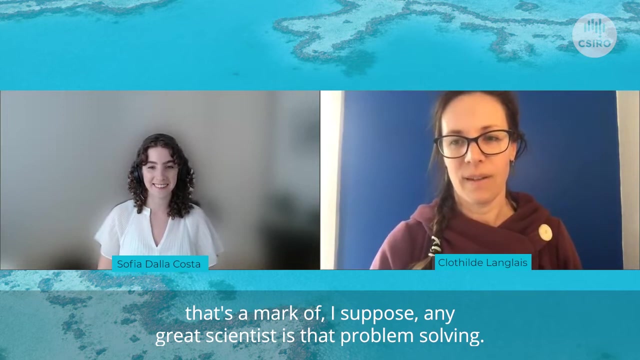 I'm still studying the circulation of the ocean because I was, I loved animals, but I was fascinating by the law of physics and how you can understand how everything works just with equations Like from that. that's a mark of, I suppose, any great scientist: is that problem solving. essentially that's what science is, isn't it? 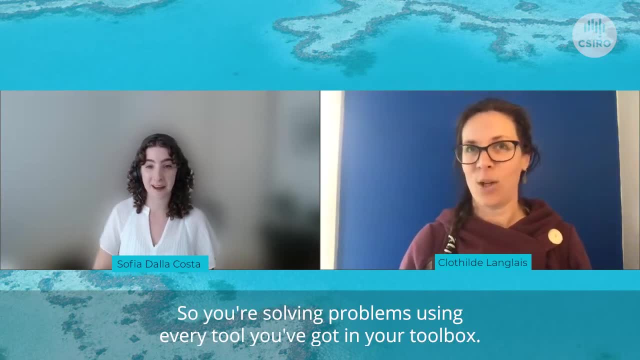 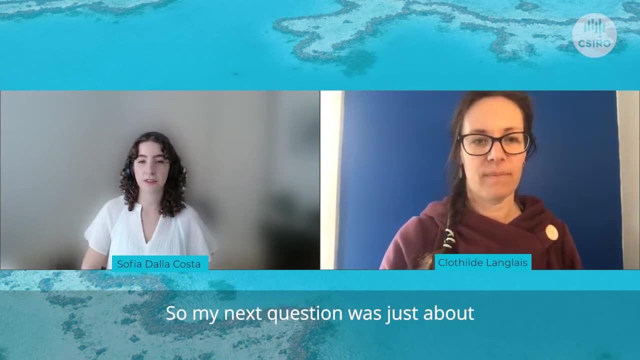 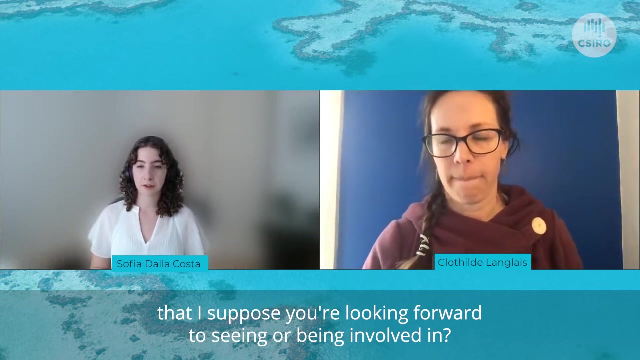 It's just solving problems. Yeah, So yeah, solving problems using every tool you've got in your toolbox? Yeah, Absolutely. So my next question was just about: is there an exciting advancement in your field that I suppose you're looking forward to seeing or being involved in? 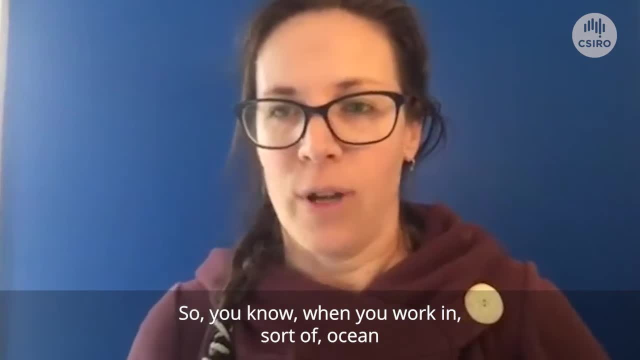 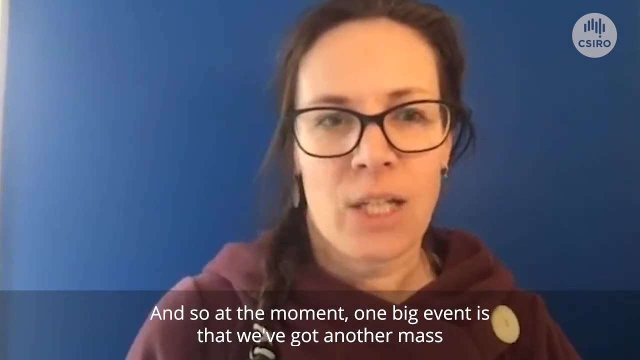 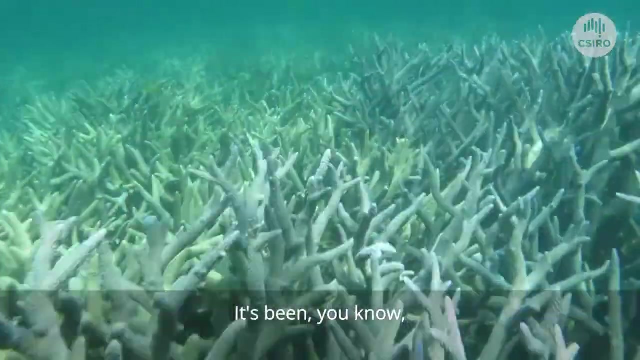 So you know, when you're working in sort of ocean climate science, it's not always super positive. So at the moment, one big event is that we've got another mass bleaching event that just happened in the Great Barrier Reef. It's been, you know, the. 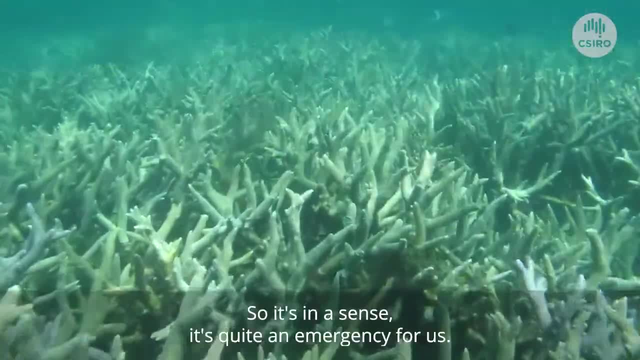 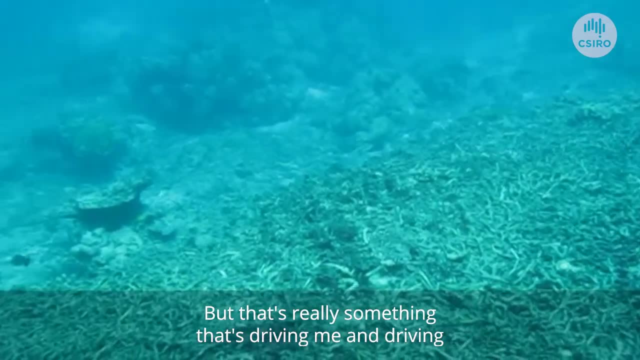 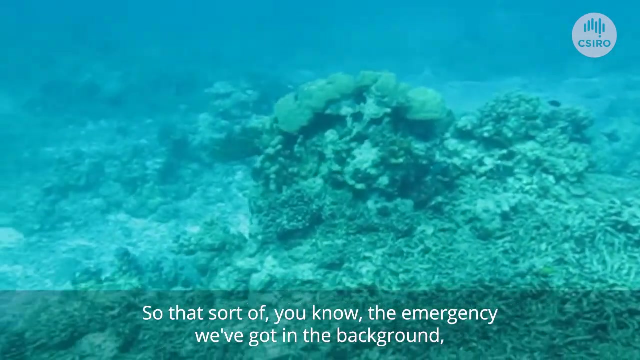 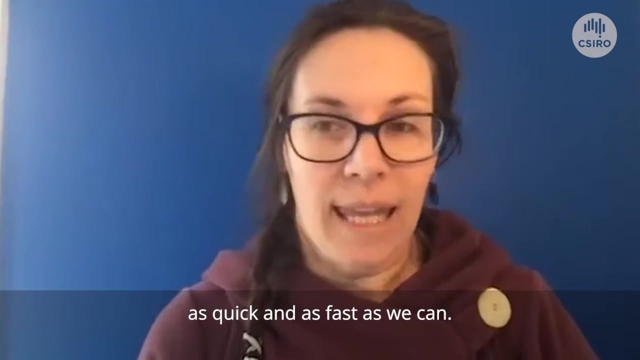 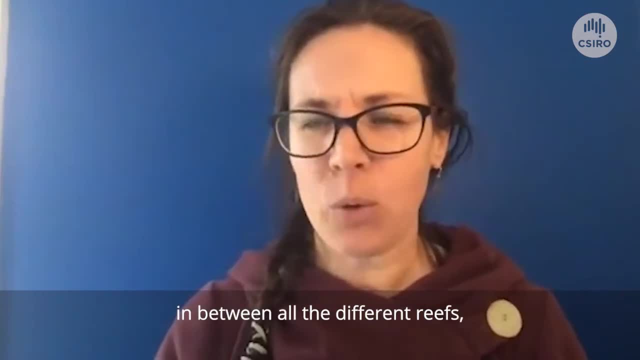 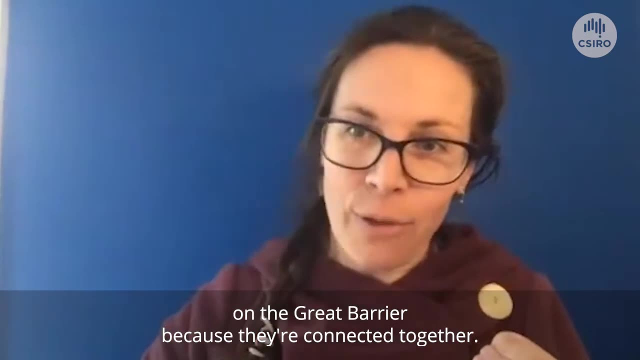 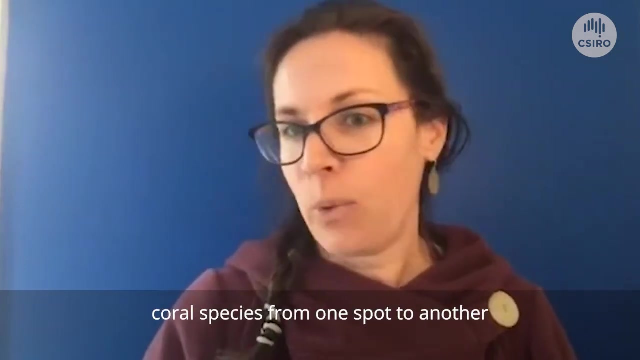 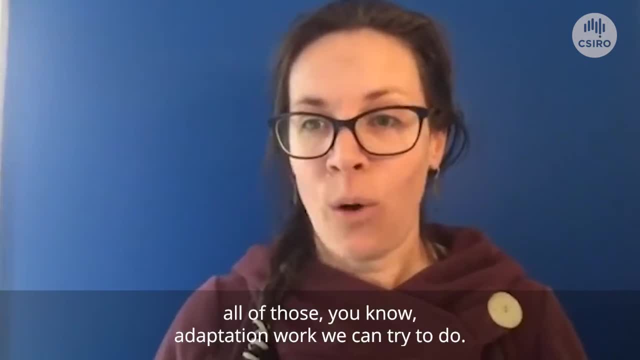 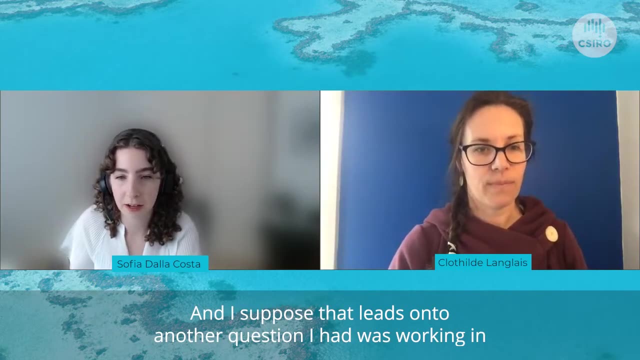 Coral species from one spot to another so they're more resilient to to heat and and all of those you know, adaptation work we can try to do Okay, And I suppose I had was just working. in the field that you are, there is a lot of, I suppose, doom and gloom. 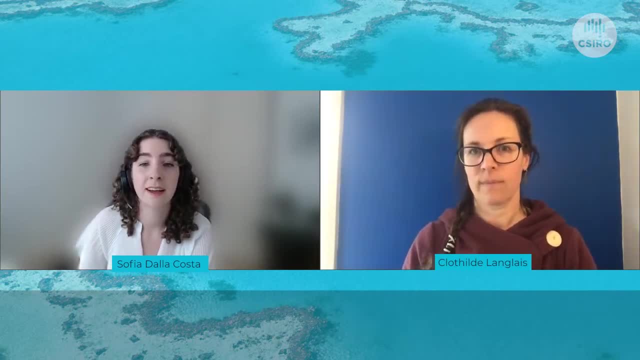 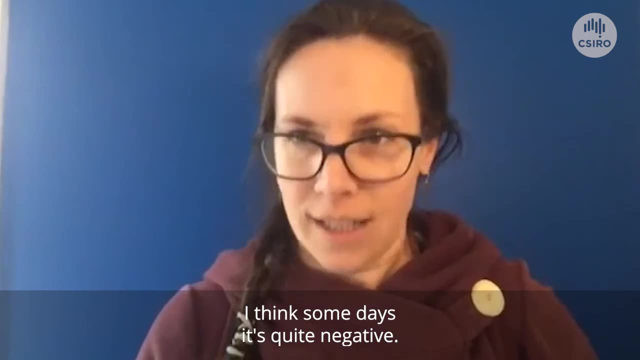 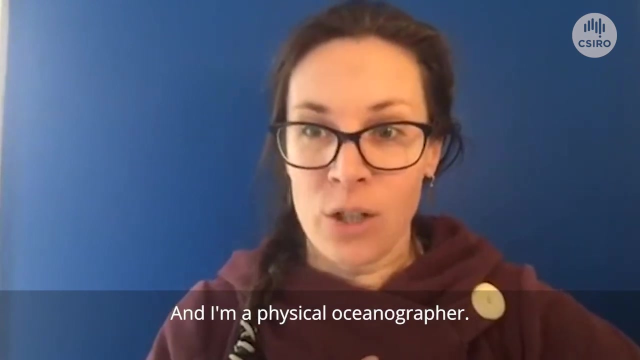 that's often um accompanies like climate change research. how do you deal with that? I think it's. it's some days it's quite negative. you're and, and, but you can only control what you can control and um, I'm a physical oceanographer. I can't control the carbon emission. 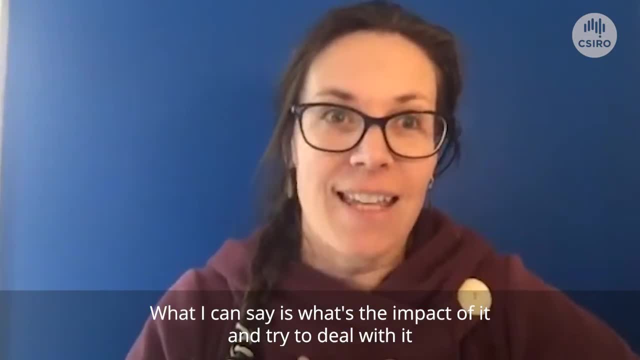 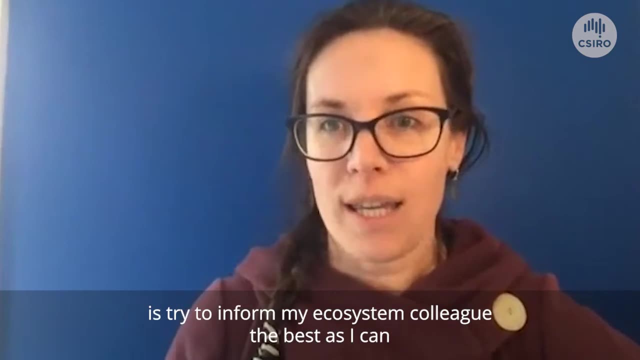 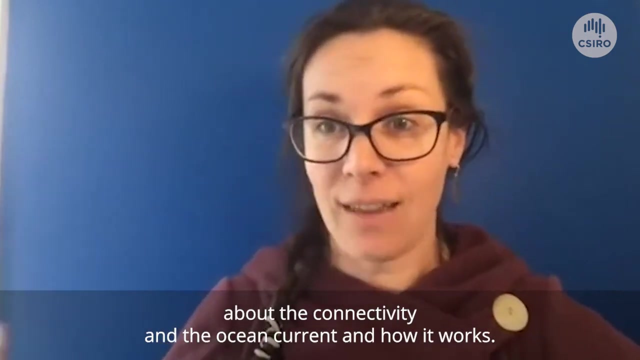 in any ways. what I can say is what the impact of it and try to deal with it the best that we can. so what I can control is um. try to inform my ecosystem colleagues the best as I can about the connectivity and the ocean current and how it work. um also, I can also inform in a 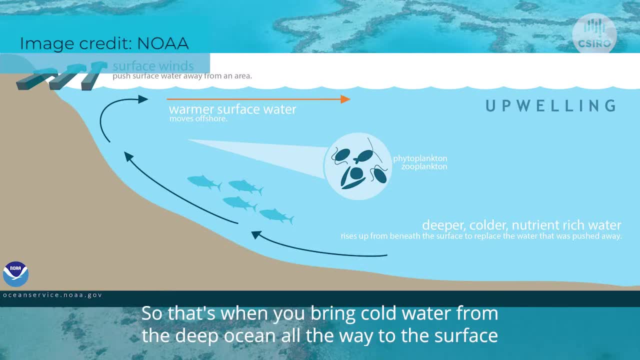 great by a reef how the upwelling are working. so that's, when you bring cold water from the deep ocean all the way to the surface, and somehow those upwelling they work with the wind and they work with the tides. so it's, it's not. 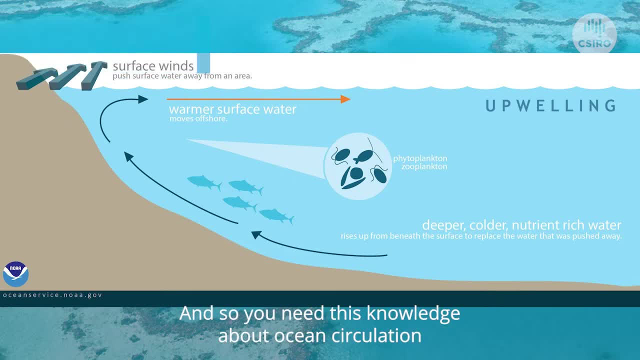 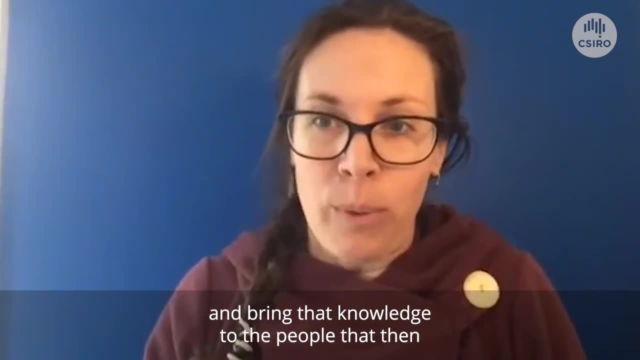 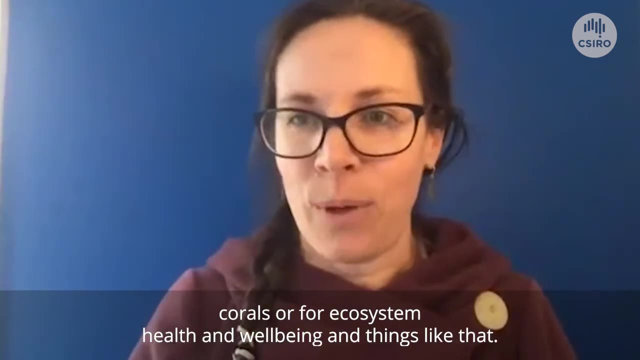 an easy process to understand. um, so you need this knowledge about ocean circulation to understand where they happen and how strong they are, and bring that knowledge to the people that then can use this information for down the track for moving corals or for ecosystem health and well-being and things like that. so, really focusing on what I can do rather than yeah. 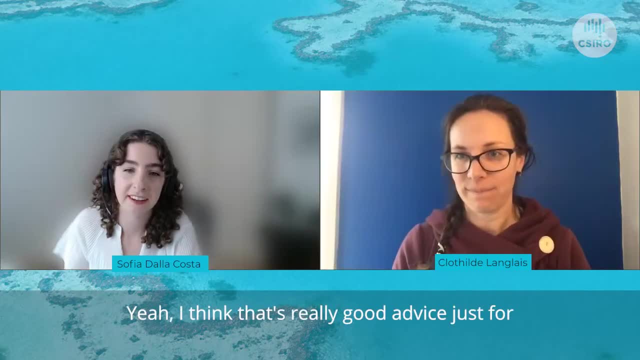 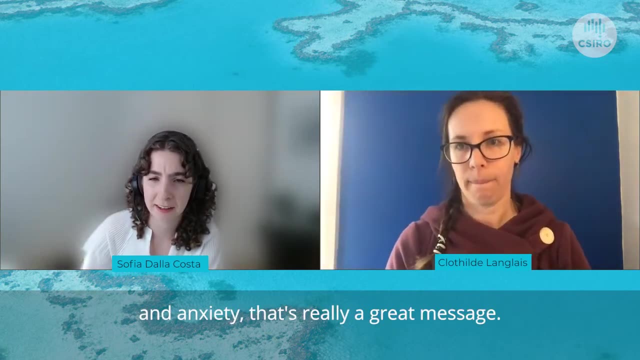 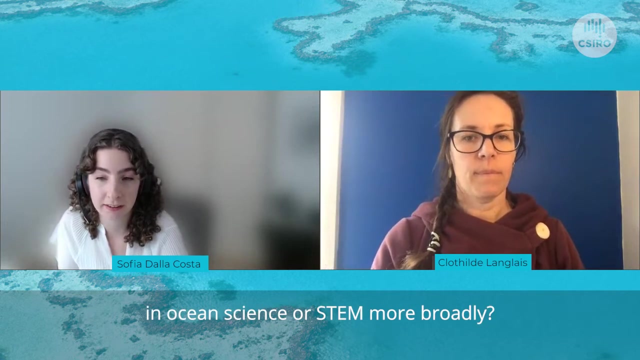 still, that is out of my control, really, yeah, I think that's really good advice just for, um, I suppose, anyone out there with the climate grief, um and anxiety, that's really a great message. what has been your experience working as a woman in ocean science or stem more broadly? 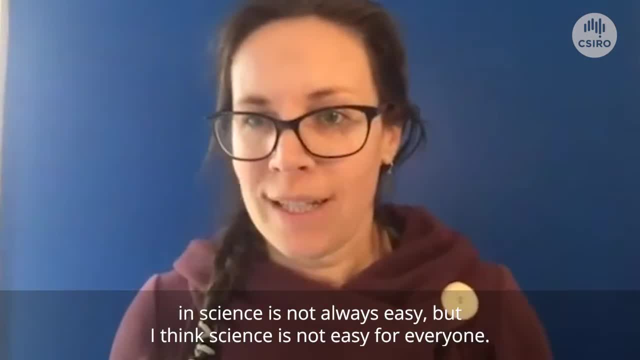 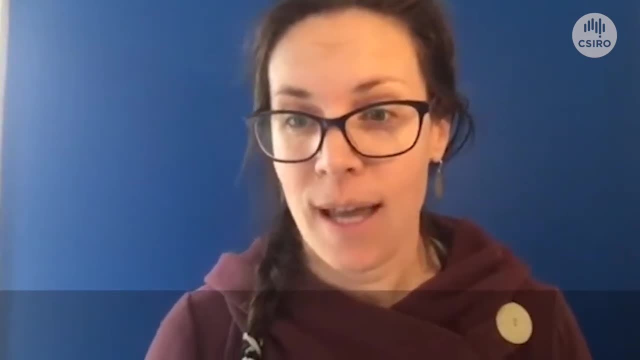 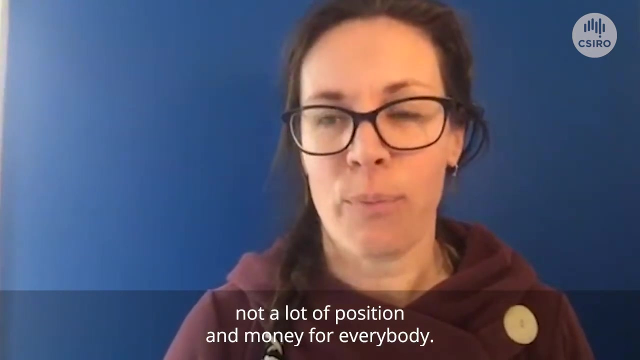 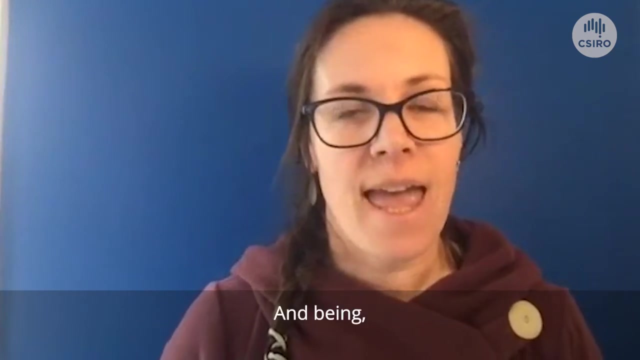 well, being in a woman in science is not always easy, but I think science is not easy for everyone. actually it can be a very tough environment, um, it can be highly competitive and they're often, you know, not a lot of position and money for everybody. so that's where the competition come in um and be, you know, very competitive. 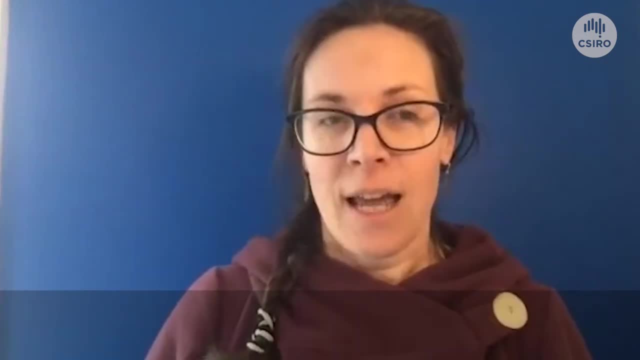 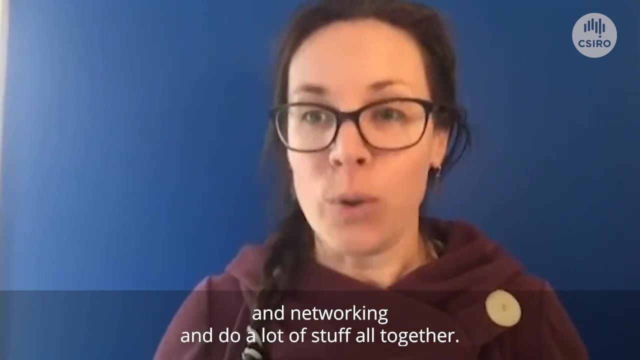 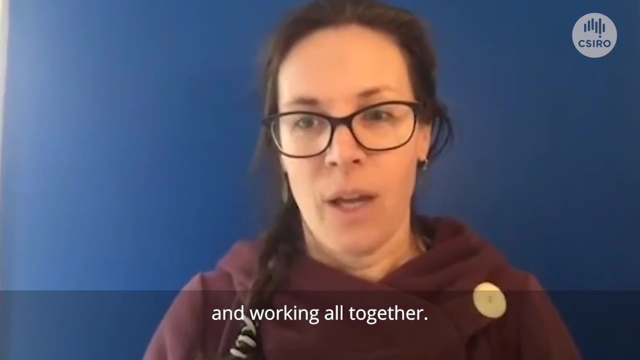 is not often a woman strength. uh, for me, a top value would be more collaboration and networking and do a lot of stuff all together, and sometimes it's a bit counter-intuitive when you think about competition and working all together, but a good thing about science is that 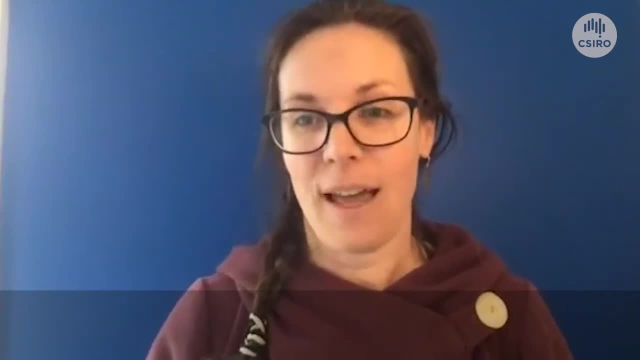 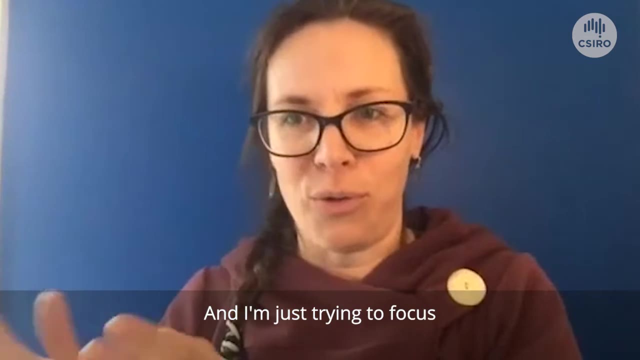 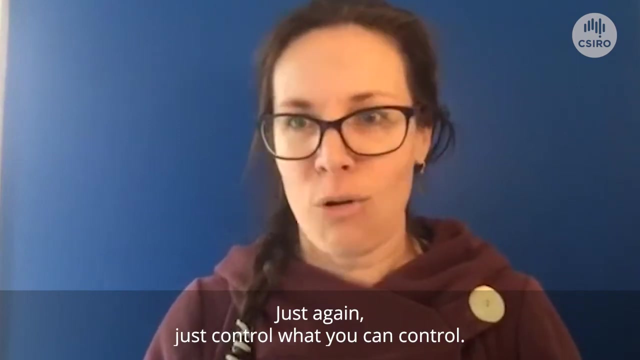 you need collaboration to move forward. um, and that's what I'm trying to focus in on. I'm trying to not too much focus on competition side of things and I'm just trying to focus on networking and collaboration, and I think that's how you move forward. just again, just control what you can. 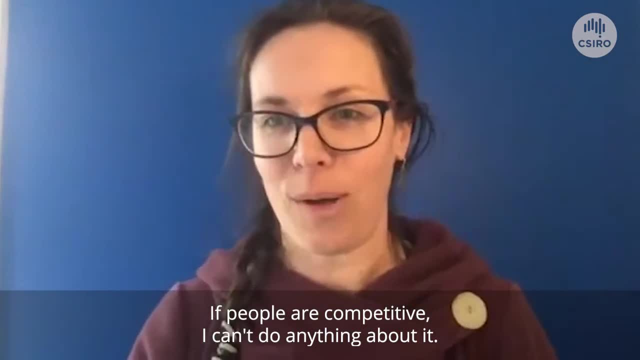 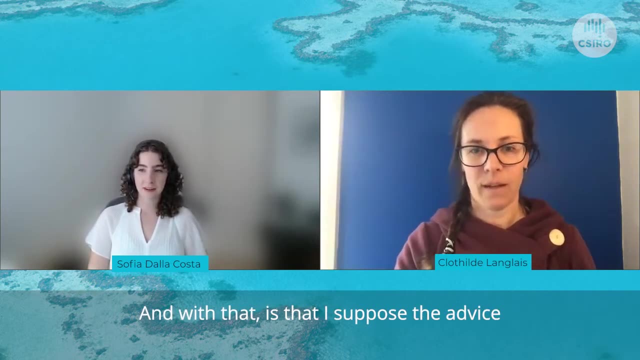 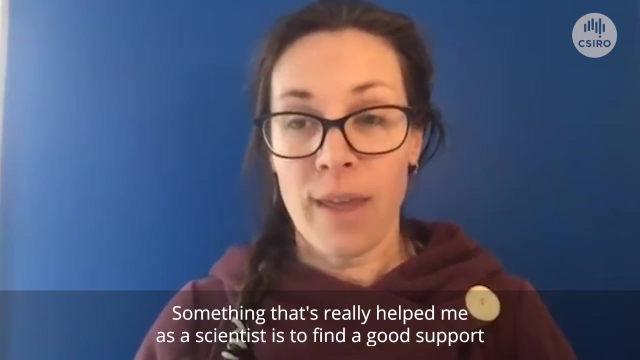 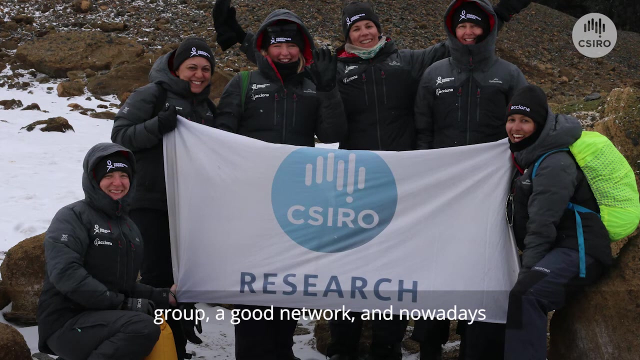 control if people are competitive, I can't. I can't do anything about it. however, I can be collaborative in my own ways. yeah, absolutely, and with that is that I suppose the advice you would give women looking to go into ocean science. something that really helped me as a scientist is to find a good support group, a good Network, and and and- nowadays there's a lot. 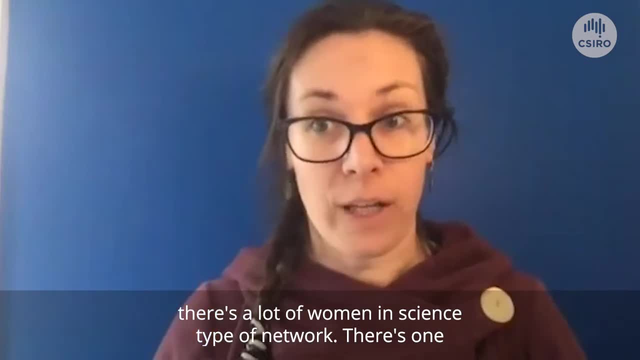 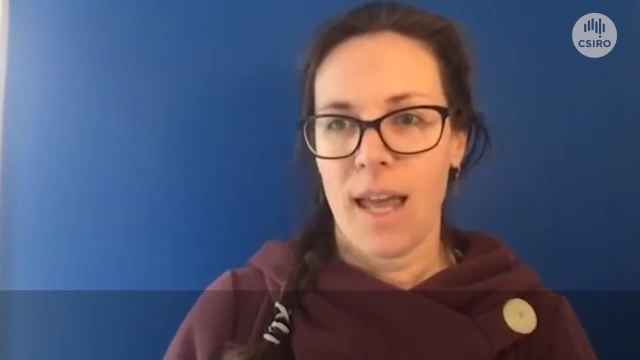 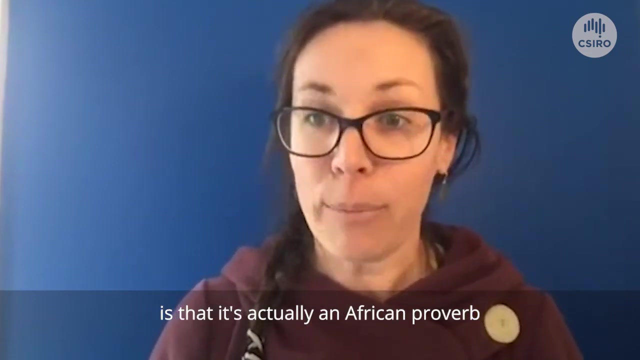 of women in science type of Network. um, there's one for the Great Barrier Reef. it'd be the, the woman in the Great Barrier Reef Network. you know, and and there's a good proverb that we've got going around in those group is that it's a, actually an African proverb. that means if you want to go fast, you go. 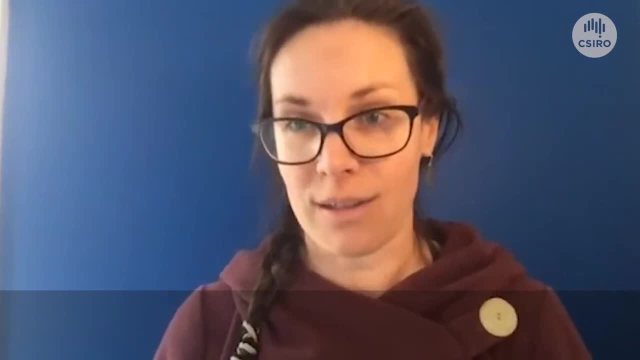 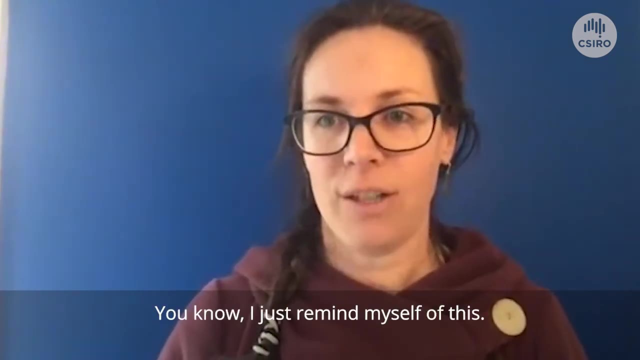 alone, but if you want to go far, you go with others, and that's something I kind of remind myself each time that I found things that are a bit tough. you know, I just remind myself of this. we're stronger together and, if needs be, I go back to my 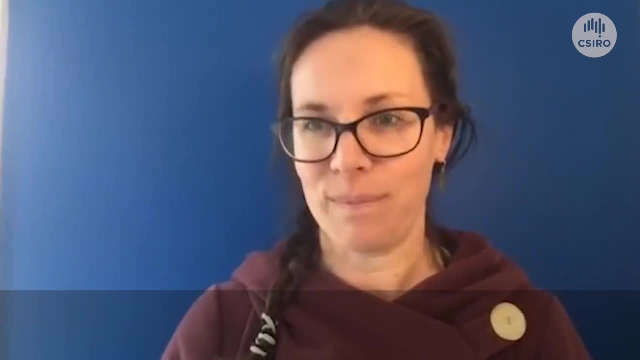 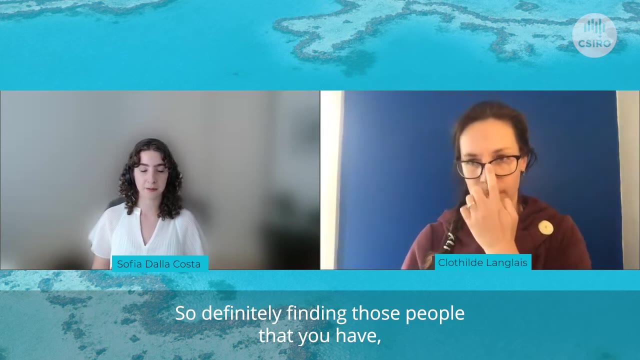 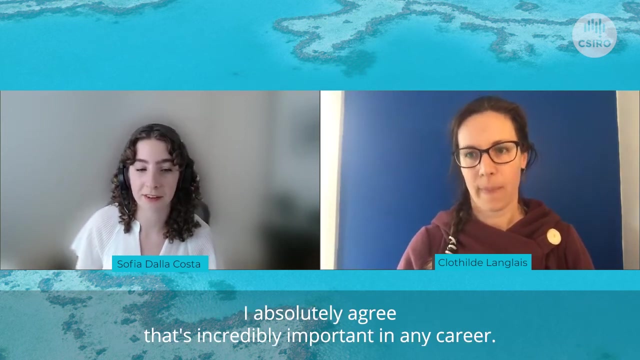 my support group and ask for advice and and support. that's really lovely. a support group is a really important part and it's so valuable. so definitely finding those people that you have, um, you know, like-minded friendship group and a support Network, I would absolutely agree that's. 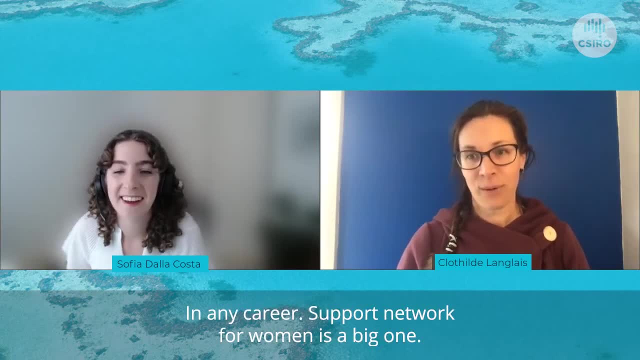 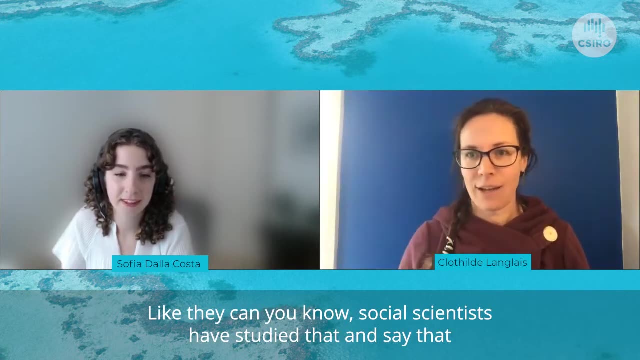 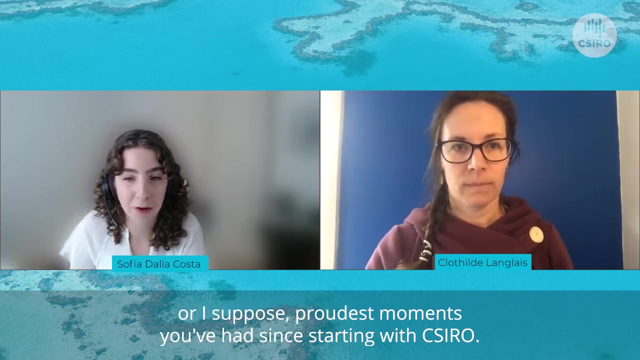 incredibly important in any career, in any career support Network for women is a big one, like they can. you know. social scientists have studied that. say that when people got a network support behind them, they do better in science. that's incredible to hear, and I wanted to ask about one of your favorite or, I suppose, proudest moments you've had. 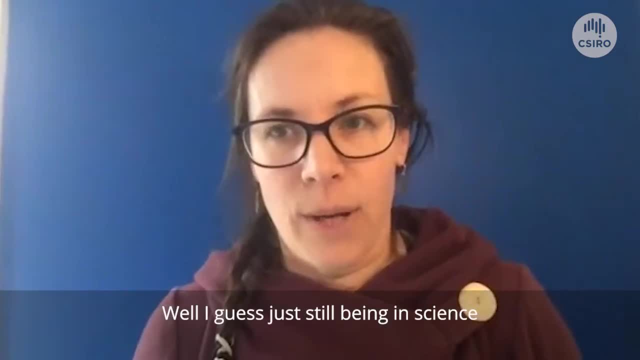 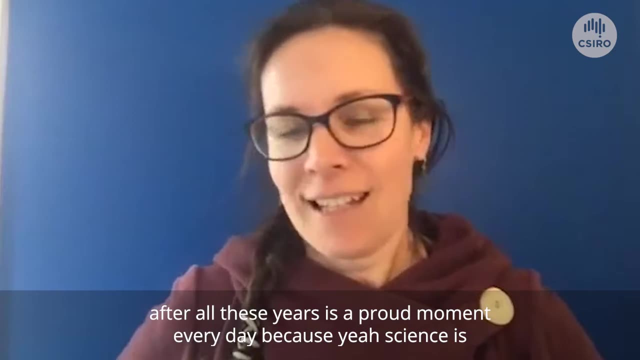 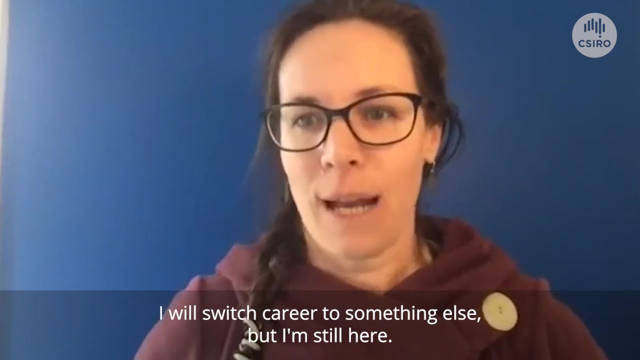 starting with CSIRO. well, I guess just still being in science after all these years is a proud moment every day, because, yes, science is tough and it's been some times where I thought I will switch career to something else, but I'm still here and so I'm just proud to be here and and try to do my 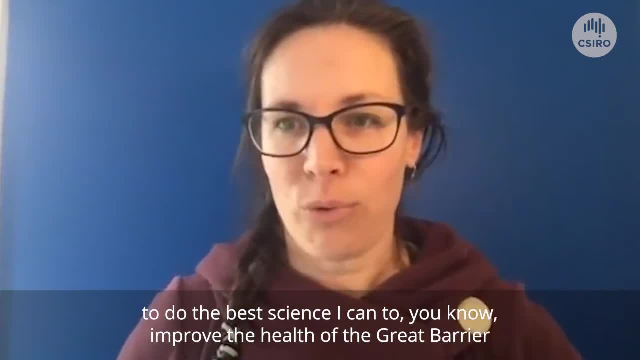 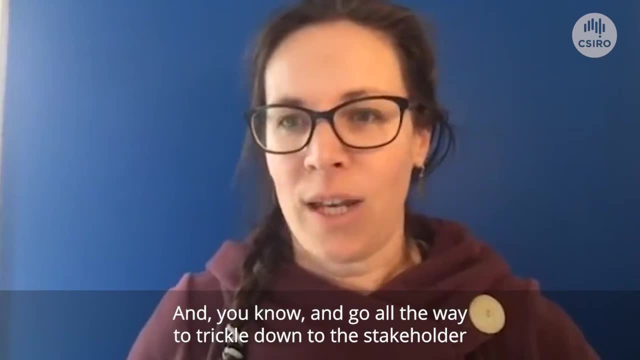 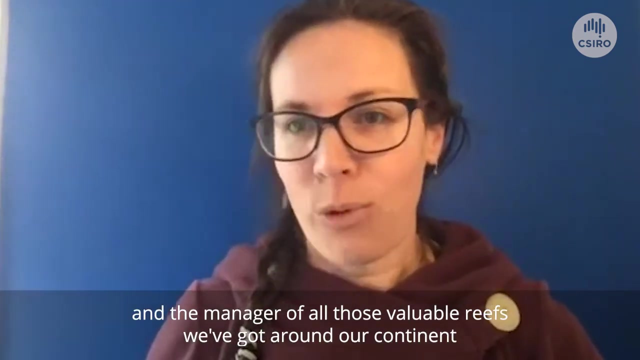 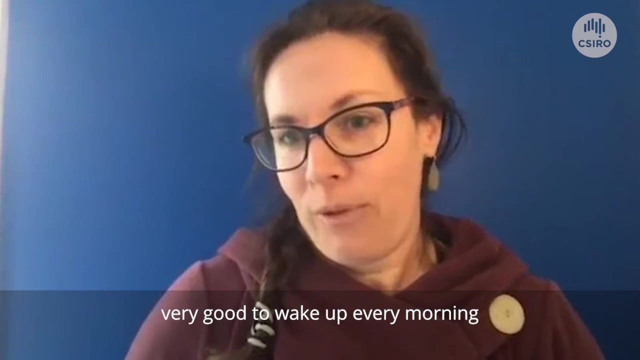 best to do the best science I can to you know, improve the health of the Great Barrier Reef, or improve that knowledge of circulation around Tasmania, and you know, and go all the way to trickle down to the stakeholder and the manager of all those valuable reef we've got around our continent. it's just you know very good to wake up every.